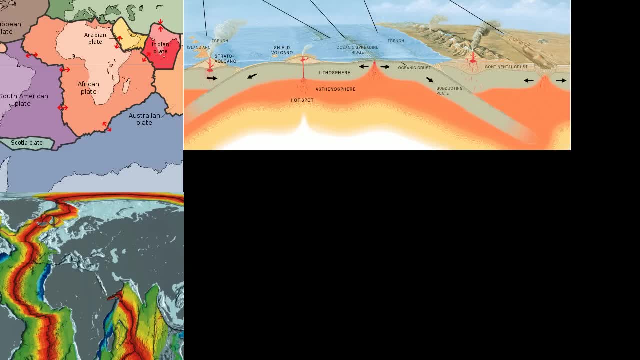 What I want to do in this video is talk a little bit about, maybe, why the plates are actually moving in the first place, And nothing I'm talking about in this video has been definitively proved. This is just kind of the current thinking, the leading thinking, on why plates are actually moving. 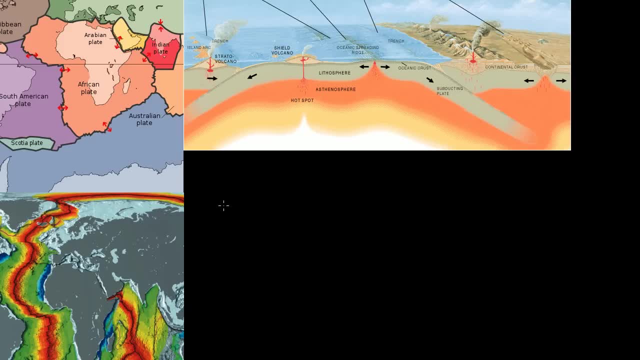 although we haven't seen the definitive evidence yet, and it's probably a combination of a bunch of things. Now, before we even talk about plates, let's just talk about convection, And you might already be familiar with the term, but just in case you're not, 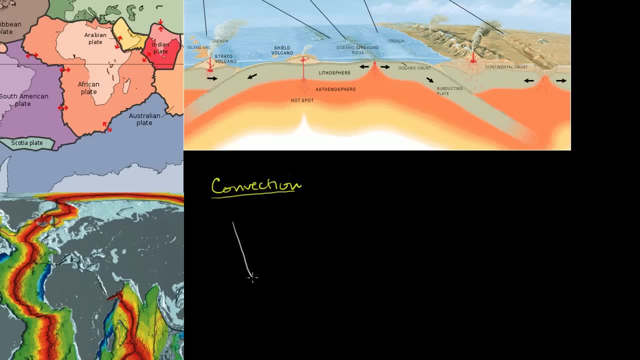 let's do a little bit of review of convection. So let's say I have a pot over here, So that is my pot and it contains some water. So I have water in my pot And let's say I only heat one end of the pot. 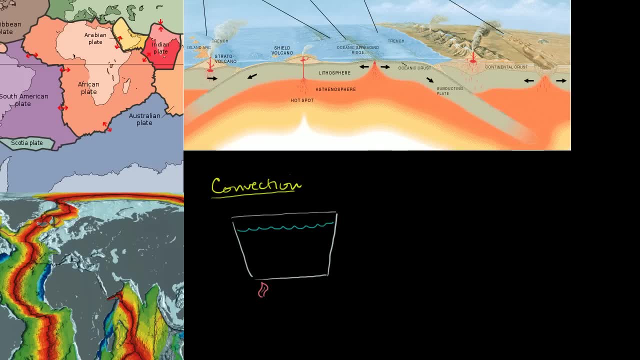 So I put a flame right over at that end of the pot. So what's going to happen? Well, the water that's right over the flame is going to be warmed up more than any of the other water, So this water is going to get heated. 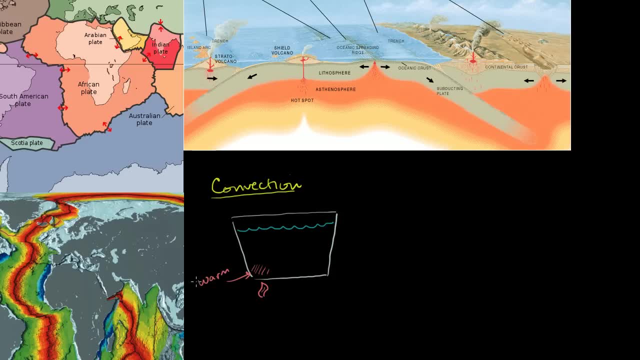 It's going to get warm, But when it gets warm it also becomes less dense. When you have a fluid, if you warm it up, the molecules are vibrating more. They have more kinetic energy. They're going to bounce further distances away from each other. 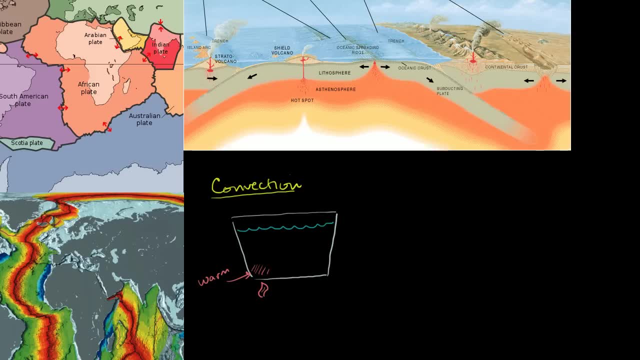 They will become less dense. And if you have something that's less dense and it's surrounded by things that are more dense- and we're dealing in kind of a fluid state right here- that warm, less dense water is going to move upwards. 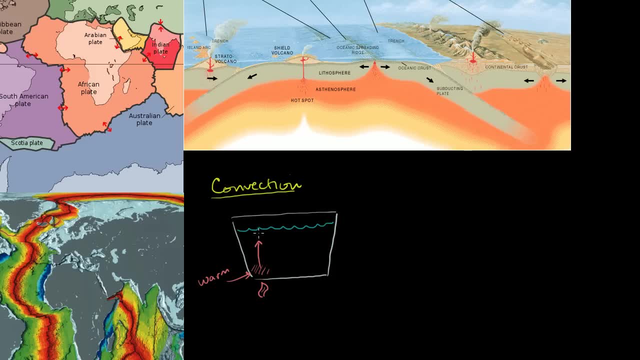 It is going to move upwards. Well, when it moves upwards, something has to replace it, Something has to replace it. So you're going to have cooler water, cooler water from this side of the container, kind of replacing where that water was. 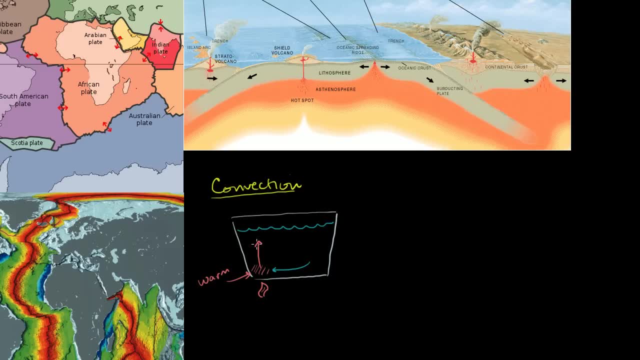 Now this water, as it rises. as this water rises, what's going to happen to it? What's going to cool down? It's going to get further from the flame. It's going to mix with, maybe, some of the other water or some of the other water, or transfer some of its kinetic energy to the neighboring water. 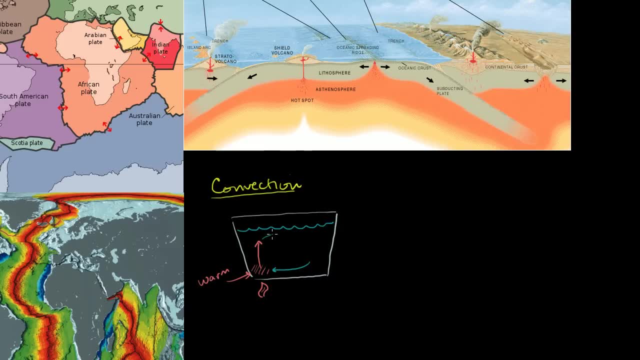 So it'll cool down. But once it cools down, what's it going to want to do? Remember, in general, the closer you are to the flame, So the water closer to the flame in general is going to be warmer, So all of this stuff is going to be warmer. 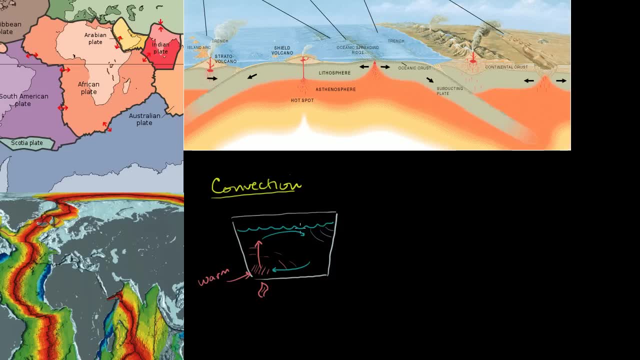 And all of this stuff up here, like the coldest water is always going to be furthest from the flame, And so it's going to be. the coldest water is going to be over here, But remember, the coldest water is also the densest water. 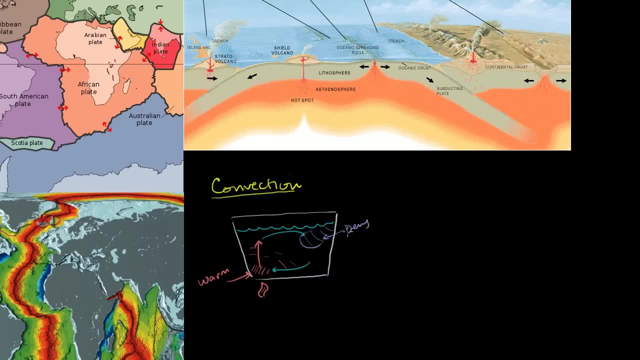 So this water over here is dense, And so it will sink. It's denser than the water around it, And it also helps replace the water that's going here to get warmed up again, And so what you do is you have this cycle here. 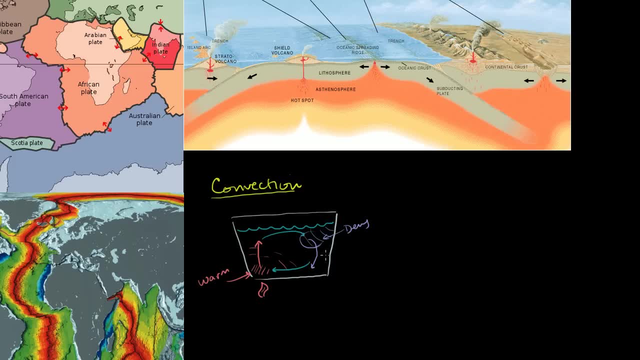 Warm water rises, moves over to the right down here and then goes back down as it cools down And it's dense And then it gets warmed up again. And so this process, essentially what it's doing is it's transferring the heat. 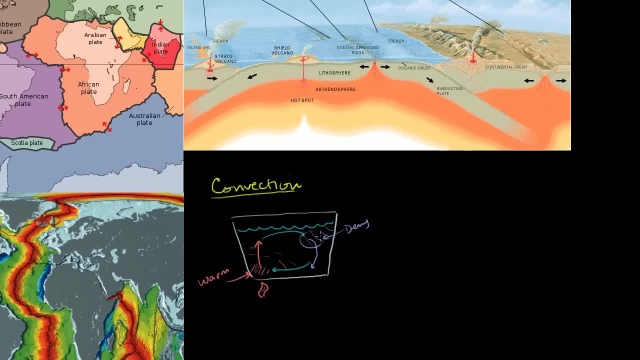 It's allowing the heat to be transferred from this one spot throughout the fluid, And so we call this process this is convection. Now, the reason why we think the plates are moving is because we think that there are similar types of convection cards in the asthenosphere. 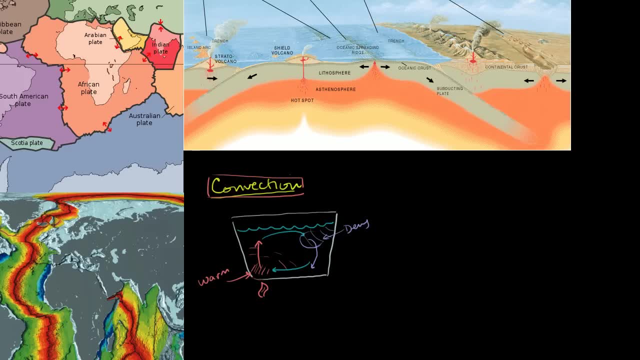 in the mantle, in the more fluid part of the mantle, Remember the mantle. most of the mantle is kind of this: you can kind of view it as this mushy, spongy, not quite liquid but not quite solid state kind of plastic. 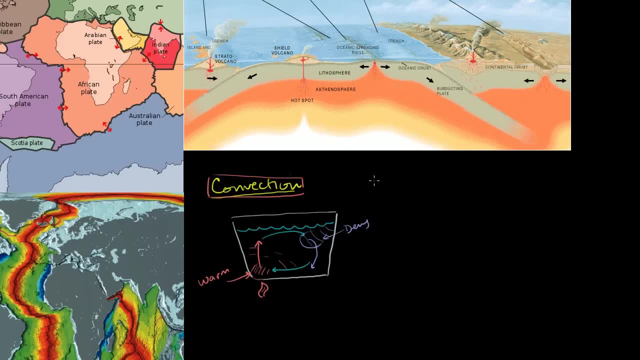 It can kind of mush past, It can kind of flow like super, super, super thick. you know. I guess you could call them, you know, like well, like super viscous fluid, so not quite solid, not quite liquid. 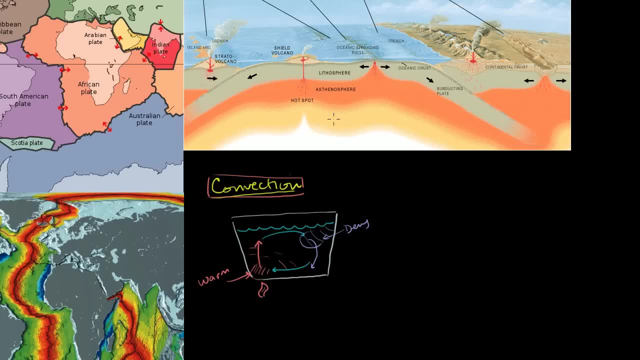 But the same thing could be happening. You have certain areas in the mantle that are hotter than others, and it's particular in the asthenosphere And those areas. that's where you're going to have, that's where you're going to have the material in the mantle move up. 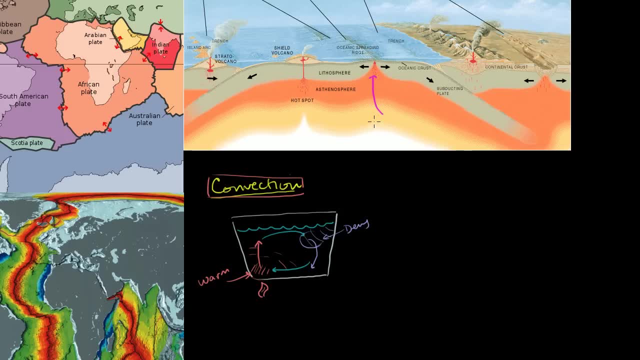 because it's hotter, it's less dense and it will move up And maybe it'll cause one of these divergent rifts where content, where kind of plate material and crustal material is forming And then, as it moves up, it cools down. 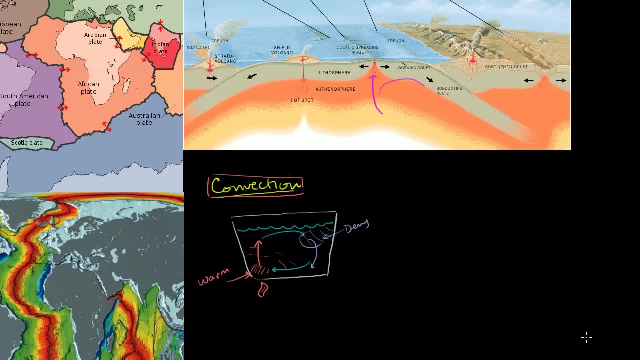 it cools down. it cools down and eventually sinks, and eventually sinks, only to get heated up again, So it has this kind of circular motion, just like we saw with the boiling water, And so that process- remember, this- isn't completely liquid.